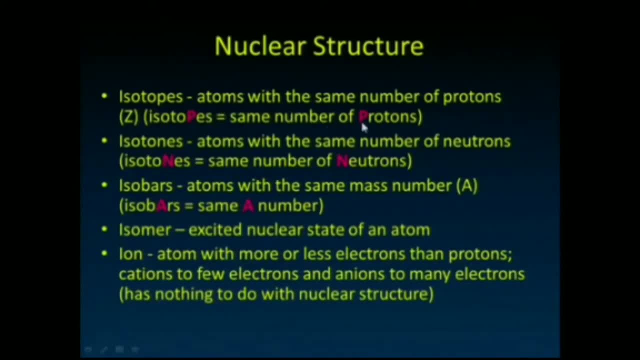 They're just going to have varying numbers of neutrons, but all have the same number of protons, And of course they're all oxygen atoms, because it's the number of protons that defines what atoms are. So we're going to talk a little bit about isotopes, which are atoms that have the same number of neutrons. 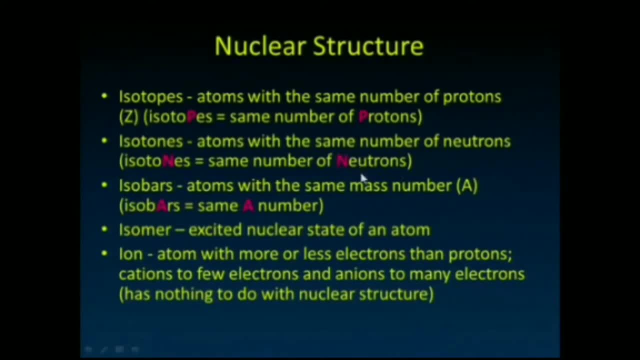 And it turns out that we can utilize some of these to create some of the radioactive elements that we're going to utilize in imaging. There's also a concept called isobars. These are atoms that have the same atomic mass number, So if you add up the number of protons plus the number of neutrons, those are the same. 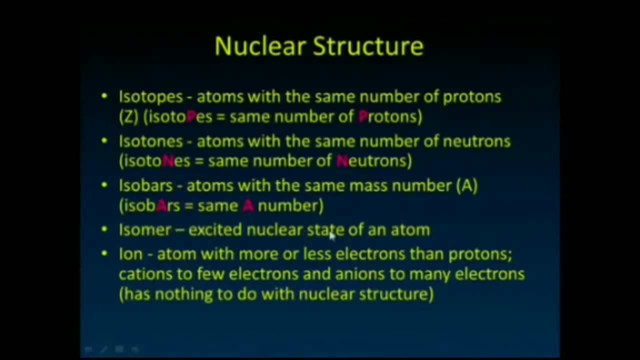 The term isomer, which is the excited nuclear state of an atom, and we're going to talk about that when we talk about isomeric transition and the gamma ray that's given off from that. And I want to distinguish all those names from the ion right, which is the atom that has more or less electrons than protons and therefore either has a positive char- a net positive charge or a net negative charge. 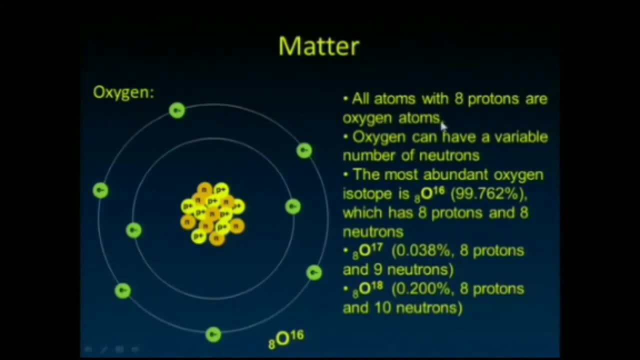 So here's oxygen, right. All atoms with eight protons are oxygen atoms, And oxygen can have a very high number of protons And oxygen has a variable number of neutrons. The most abundant oxygen isotope is 016,: eight protons, eight neutrons. 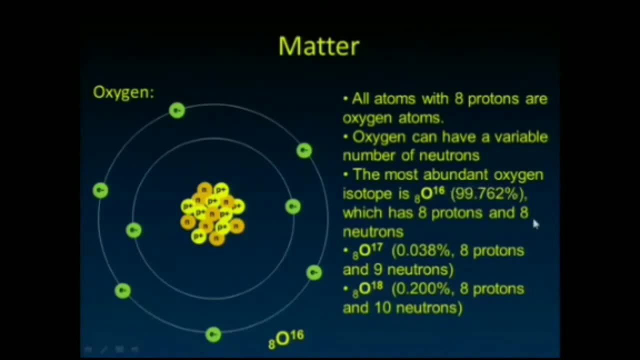 And in fact 99.762% of all naturally occurring oxygen occurs in that form. There's 017 and 018,, by the way, both of these are stable, They don't go and undergo radioactive decay, And a very small percentage of the natural occurring oxygen is in those two forms. 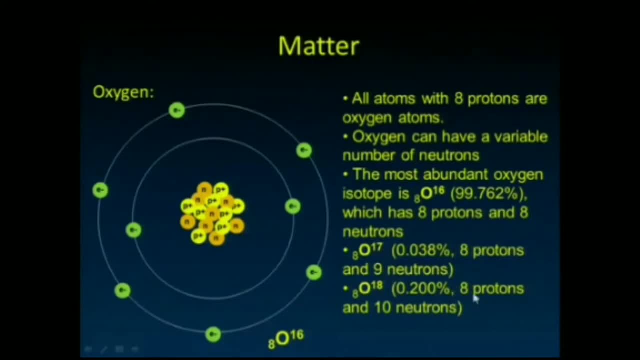 So this form with eight protons protons and nine neutrons: O18, eight protons and ten neutrons. As a matter of fact, you can use O18 to make F18, if you want that we're going to use to image in PET And I guess all you need. 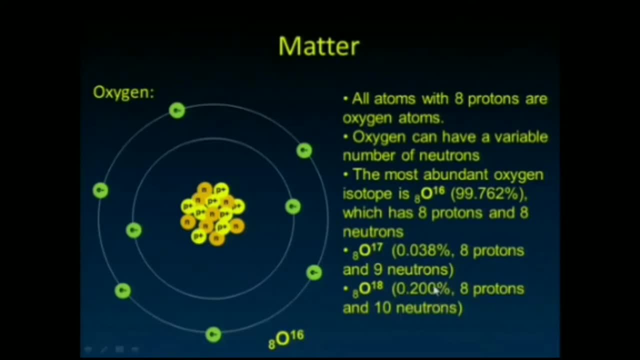 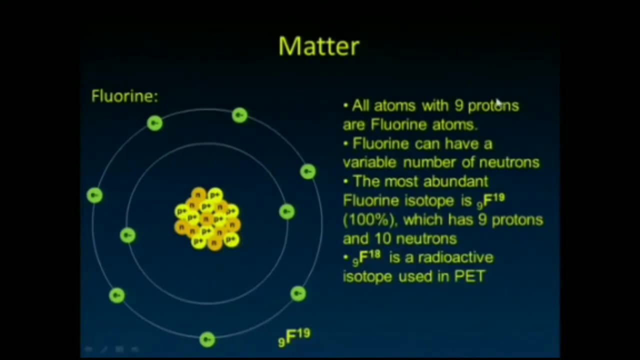 to go out and there's plenty of seawater out there right, and 0.2% of it is going to be in the form that we would need to do that. Here's fluorine. Fluorine has nine protons. It turns. 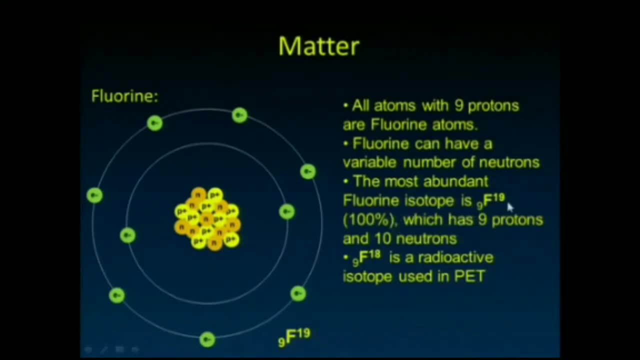 out that there's only one stable isotope of fluorine, and that's F19.. Notice: this is the first element that has an excess of neutrons to protons Up until this point, with the exception of hydrogen, which only has a proton in its nucleus right. helium: two protons, two neutrons. 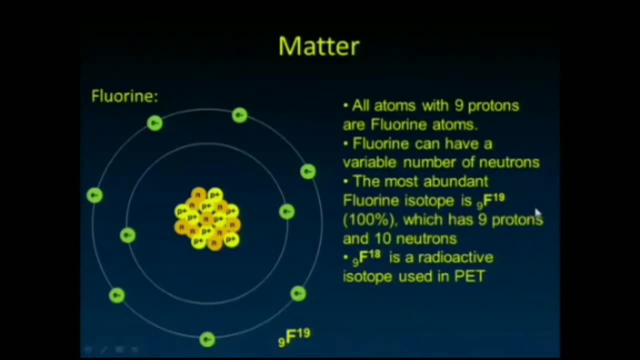 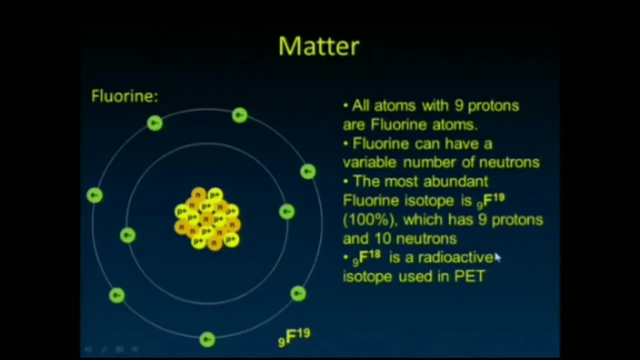 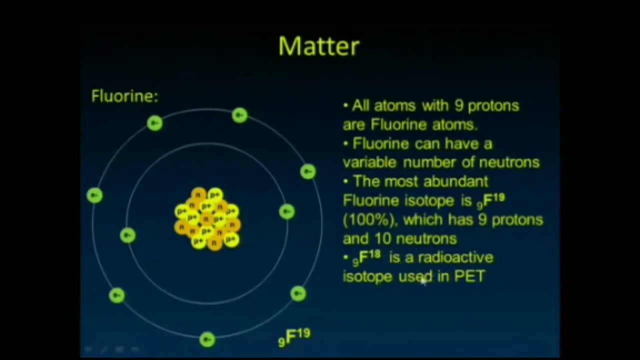 neutrons in a second F18 we're familiar with. It's that radioactive isotope used in PET. And, of course, F18 and O18, right, they're isobars of each other because they both have the sum of. 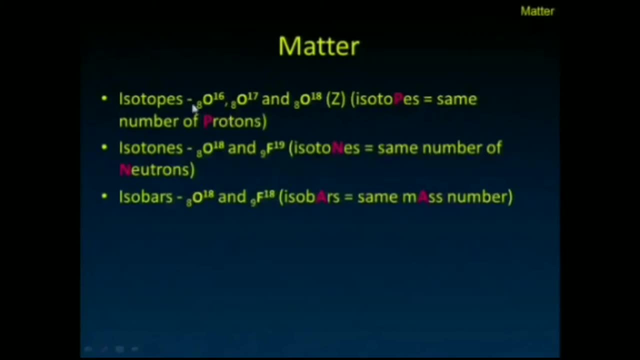 their protons plus their neutrons are the same. So here are isotopes. O16,, O17, and O18 are all protons. O18 and F19 are isotones. This has ten neutrons and this has ten neutrons And O18 and. 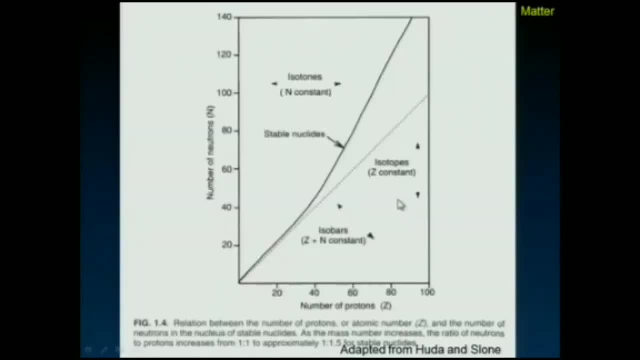 F18 are isobars, the same atomic mass number. So here's a picture from an older version of Huda and Sloan's book and I'm going to adapt it a little bit as we talk, a little bit. So as we take a look at all of the nuclei that are out there, we'll notice that there's a certain ratio. 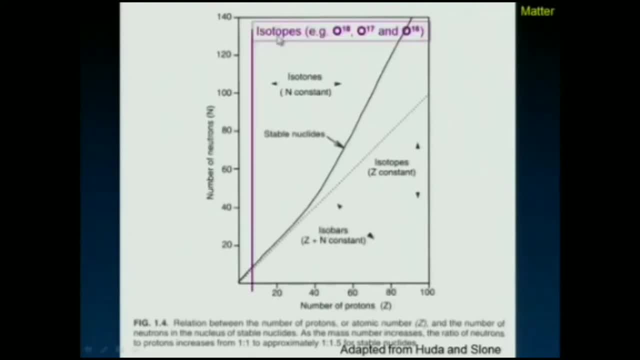 of their protons to neutrons. that occurs. But let's first kind of mark the things that we just talked about. So these vertically oriented lines are the isotopes. the things that have a constant number of protons are vertically oriented lines And I've drawn in here at about the level of eight. 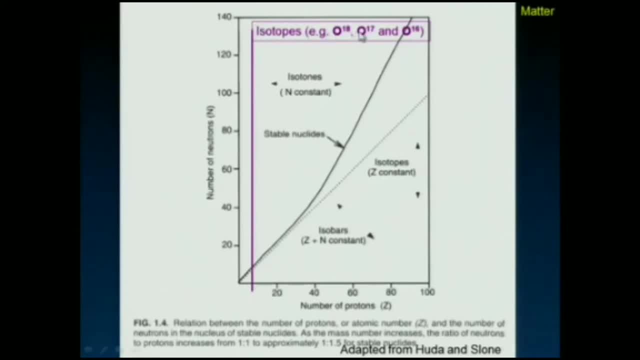 protons, the line that corresponds to where the isotopes of oxygen would fall. Here are the isotones, the things that have the same number of neutrons, And of course these would have variable numbers of protons. So there's O18,, F19, the things we talked about, And, of course, on this, 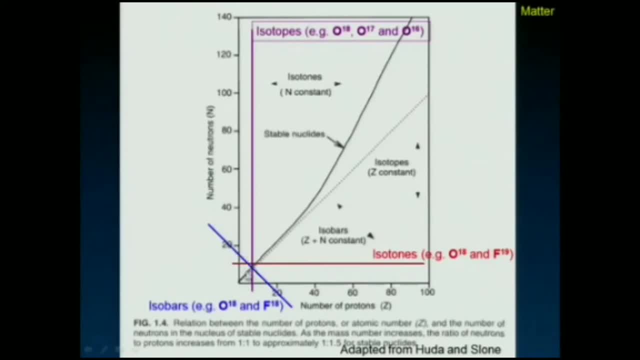 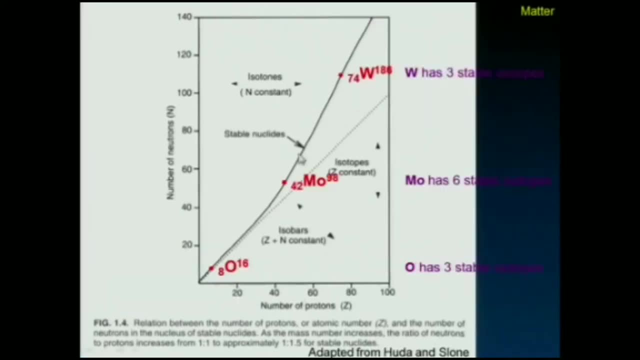 line are the isobars, things that have the sum of the protons plus the neutrons being the same. This graph shows. I've drawn some of the different atoms on this. some of the elements: Here's oxygen, O16 here. Here's molybdenum. 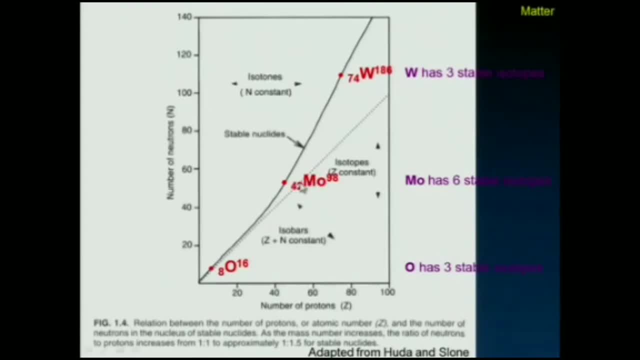 The 42nd element. it's got 42 protons And here's tungsten. We've met tungsten before with its 74 protons. It turns out, as we've already mentioned, oxygen has three stable isotopes. Molybdenum has. 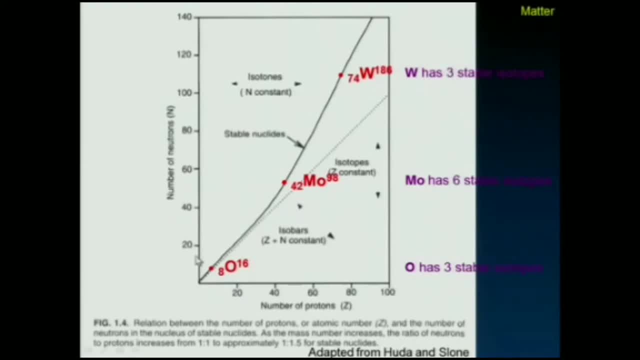 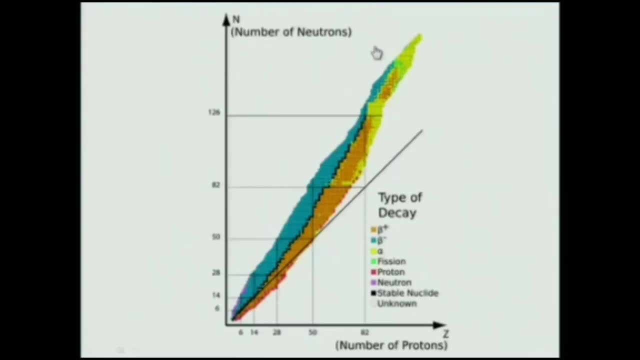 six stable isotopes And tungsten has three. So this notion that there's this simple curve of stable nuclides is really an incorrect one. This is really a better picture of how things look. The black dots on this picture correspond to the stable isotopes And the things above that black. 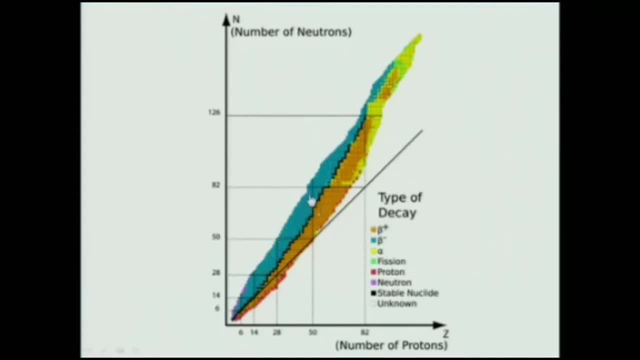 line in blue. you notice, these are the things that decay by beta minus decay, And the orange things are the things that decay by beta plus decay, And we'll talk about what that is in a little bit. And the things that are colored yellow here are things that decay by alpha decay. that we'll look. 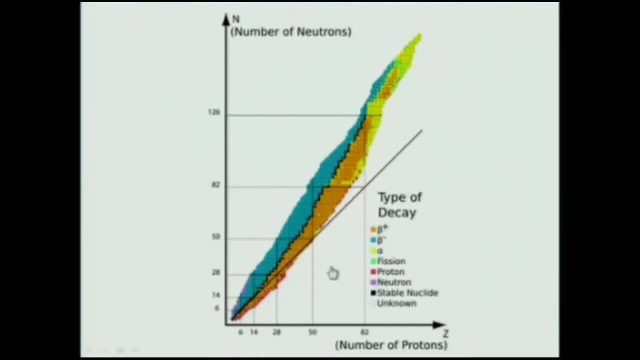 at And then down here there's a few other things that I'm not really going to get into in terms of some decay scheme, But take a look at some of the things here. For instance, here at 82,. look at how many as we go across. 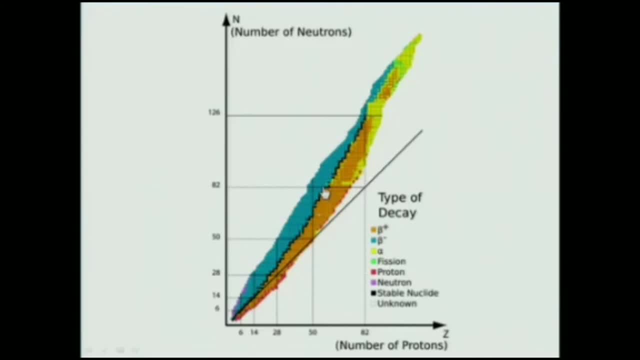 right. things are stable that have various numbers of protons but have a fixed number of neutrons there at 82.. There's a number of stable isotopes there with 82 neutrons And here's the list of them, those five things, all of which have 82 neutrons that are stable. Then also, if you'll look right, 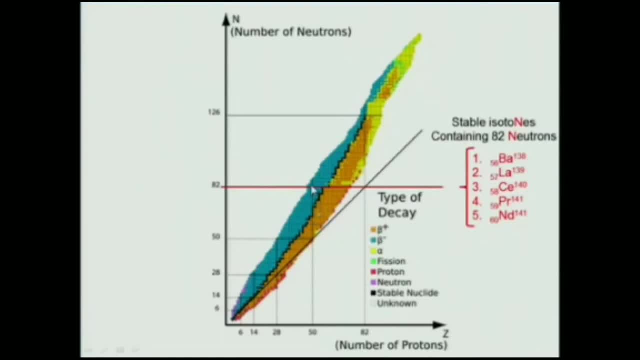 here. notice how many dark black lines there are here, right at this 50 level, right. Those are all the stable isotopes containing 50 protons. Notice how many of them there are. It turns out that that's 10.. 10 has 10 stable isotopes- by far the most here. So it's not as simple as a single curve. 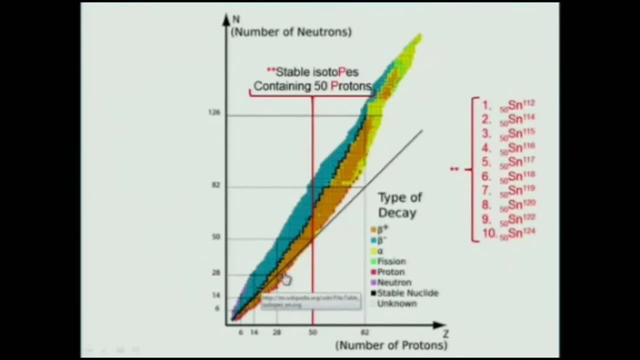 with one at each point. that does that. But there's a general trend here. Does everyone see that general trend? Right, this line, this dark line, is the line at which the number of protons and the number of neutrons would be equal to each other. So does everyone see that as the number of protons? 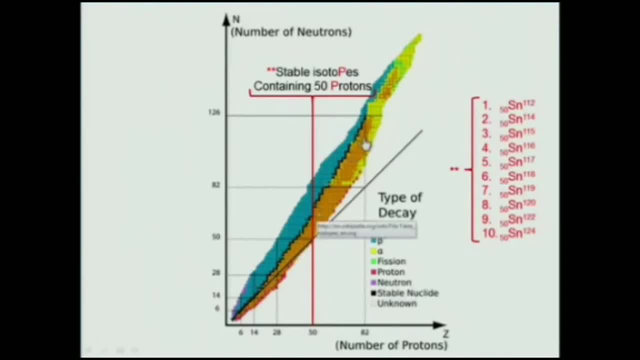 in an atom gets bigger, it turns out that you have to have a relative excess in the number of neutrons in order to have nuclear stability there right. And that's helpful to us in that we can sort of predict a little bit as to what the decay scheme might be by knowing. 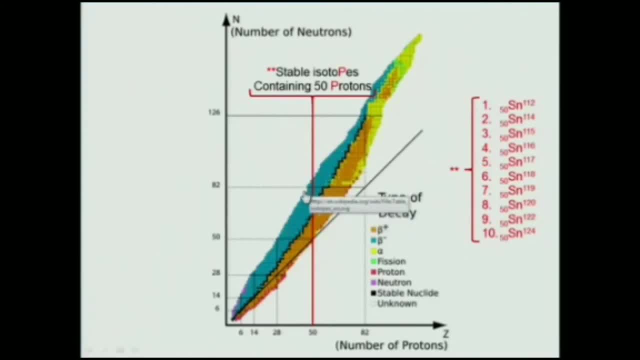 whether you exist up in this blue region- right, You have more neutrons than you need, You have an excess of neutrons- Or if you're down in this region, where I guess you would say you have either a relative paucity of neutrons or perhaps too many protons, And that's going to help us. 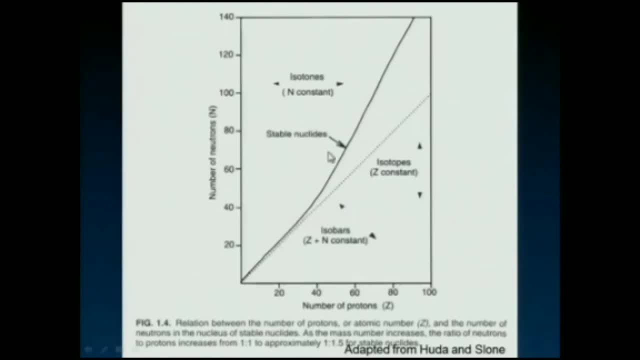 decide what the decay scheme is going to be there. So, going back to that, that picture right. These are the things that have too few neutrons, or if you will have too many protons relative to neutrons. And these are the things that have too many neutrons, or if you 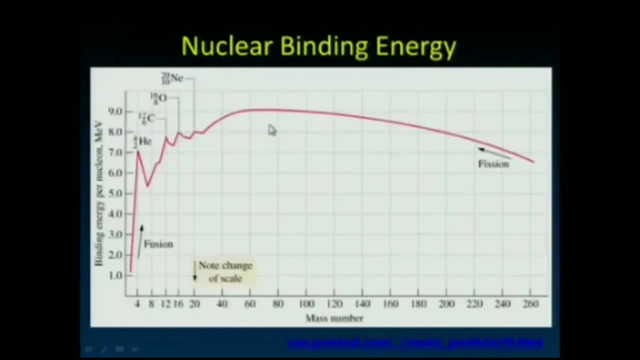 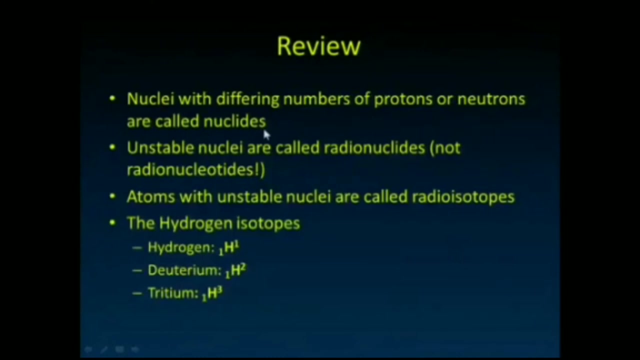 will have too few protons relative to the neutrons. there, Here's that nuclear binding energy we talked about, right, The most stable thing sitting in this range, And so things up in this range are really going to decay into that region to try and make things become more stable. 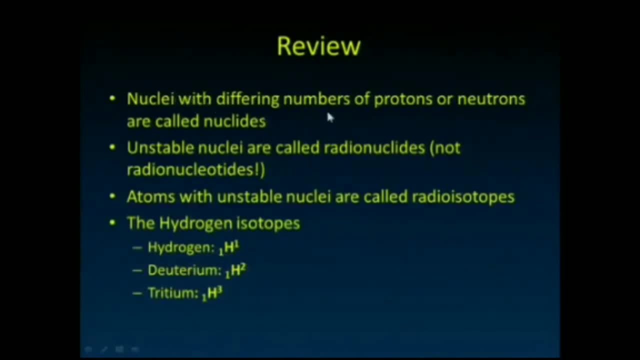 So, by way of review, right Nuclei with different numbers of protons or neutrons are called nuclides. Unstable nuclei are called radionuclides, not radionucleotides. We're not studying RNA or DNA. Atoms with unstable nuclei are called radioisotopes. So here are some of 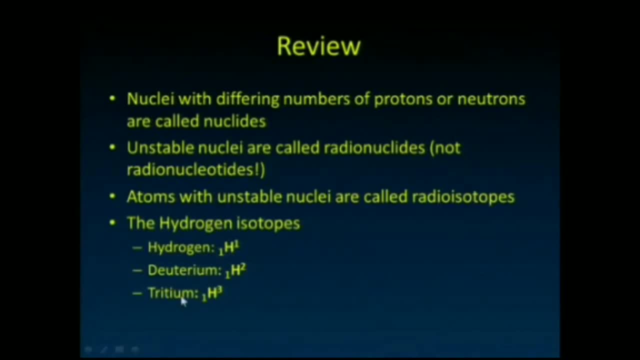 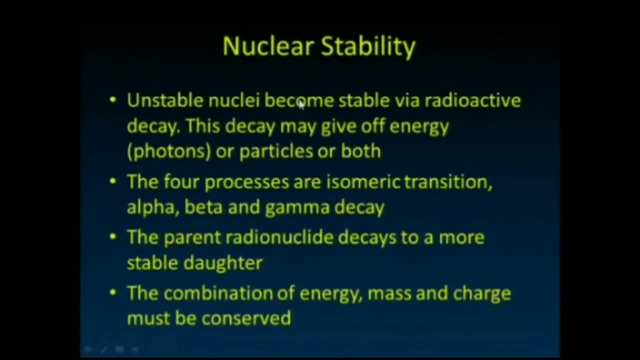 the hydrogen isotopes right Deuterium tritium. There So unstable nuclei become stable via radioactive decay. That decay may give off energy in the electromagnetic spectrum, pure energy, gamma ray, photons- or it may give off particles or, frankly, some things decay using both schemes. The four processes are isomeric.